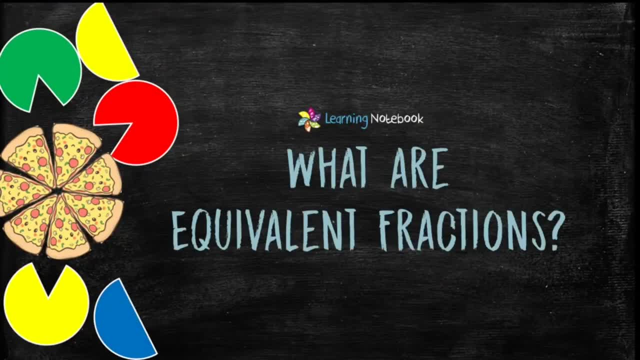 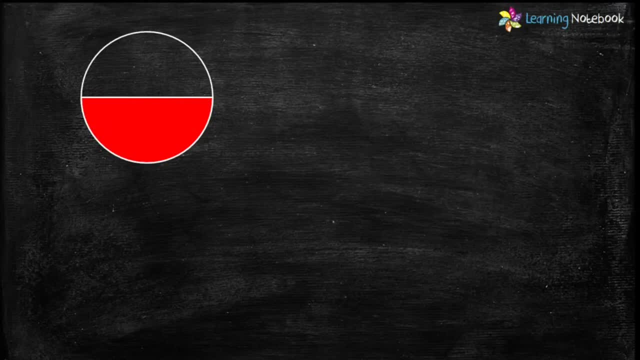 So let's start and first understand what are equivalent fractions. Students, can you tell me the fraction of colored portion in this figure? Yes, it is 1 by 2.. Now what is the fraction of colored portion in this second figure? 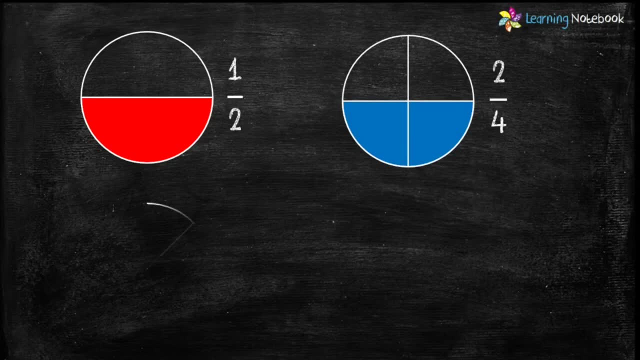 It is 2 by 4.. Next, tell me the fraction of colored portion in third figure. It is 3 by 6.. And finally, can you tell me the fraction of colored portion in this last figure? It is 4 by 8.. 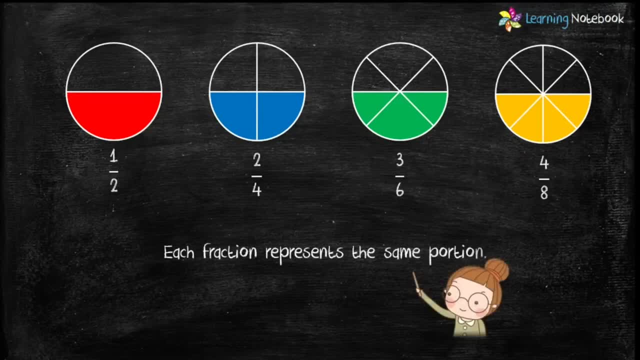 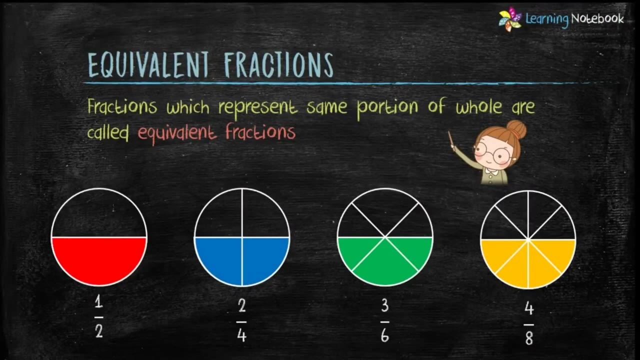 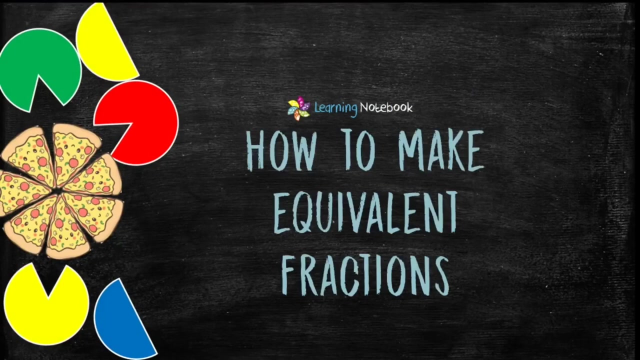 Students, did you notice that each fraction in all these four figures represents the same portion? Such fractions are called equivalent fractions By definition. fractions which represent same portion of whole are called equivalent fractions. Now let's learn how to make equivalent fractions. 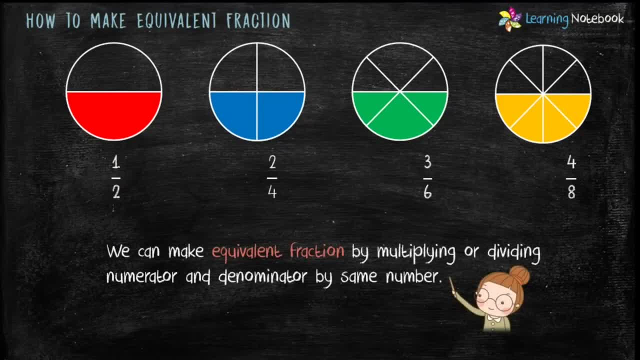 We can make equivalent fraction by multiplying or dividing numerator and denominator by same number, Like in our example: if we multiply both numerator and denominator of fraction 1 by 2 by 2, we get fraction 2 by 4.. Similarly, if we multiply both numerator and denominator of fraction 1 by 2 by 3,, 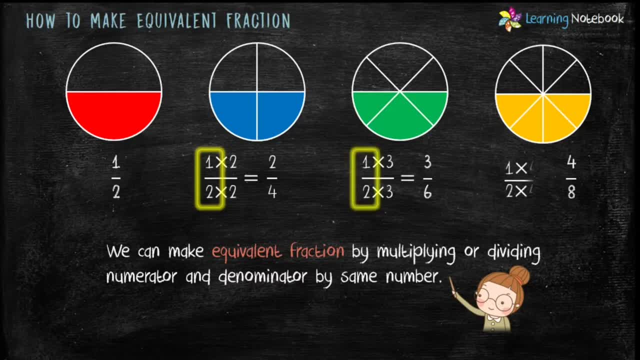 we get fraction 3 by 6.. In the same manner, by multiplying numerator and denominator of 1 by 2 by 4, we get fraction 4 by 8.. So, students, in this way we can make equivalent fraction by multiplying or dividing numerator and denominator by same number. 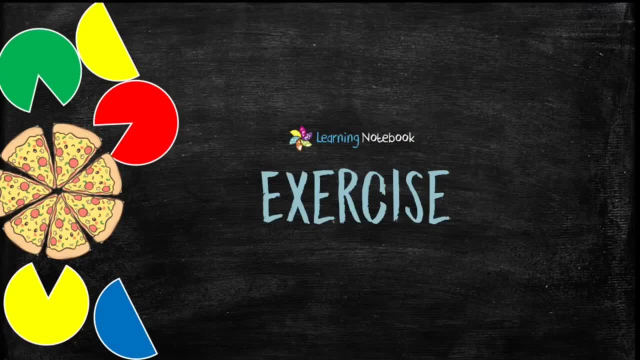 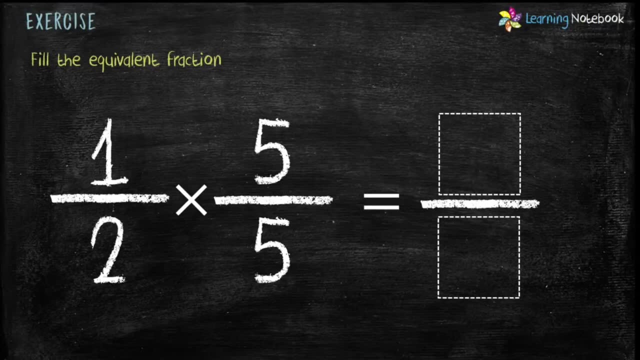 Now let's do an exercise. Fill the equivalent fraction Here. numerator and denominator of fraction 1 by 2 are getting multiplied by same number, 5.. So let's first find the numerator 1 into 5, equals to 5, and denominator would be 2 into 5, equals to 10.. 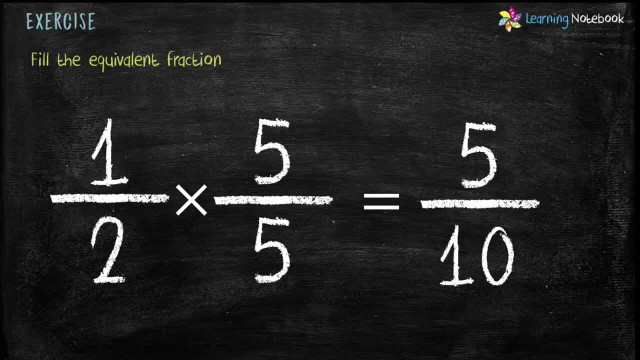 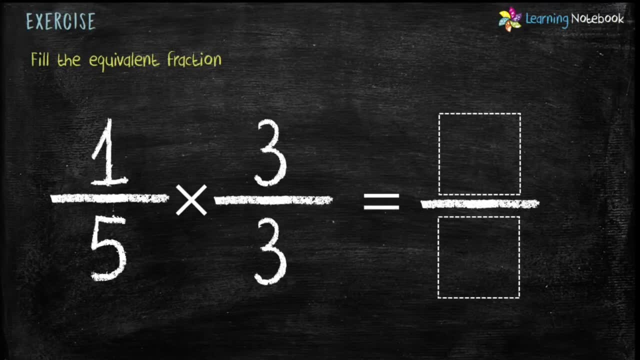 So equivalent fraction is 5 by 10.. Now let's see the next example. Students, here, numerator and denominator of fraction 1 by 5 are getting multiplied by same number, 3.. So let's first find the numerator. 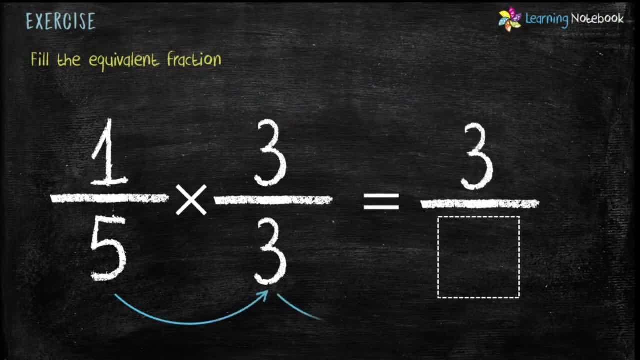 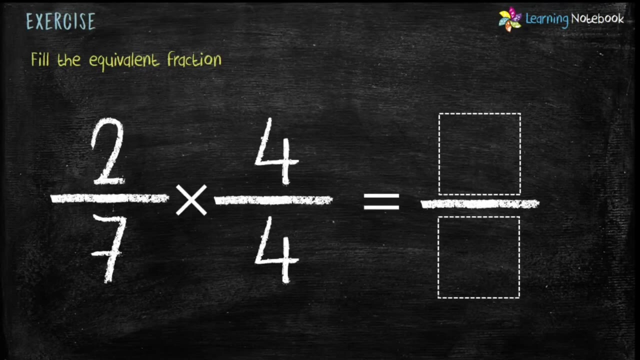 1 into 3 equals to 3, and denominator would be: 5 into 3 equals to 15.. So equivalent fraction is 3 by 15.. Now next example is 2 by 7.. Here numerator and denominator of fraction 2 by 7 is getting multiplied by same number, 4.. 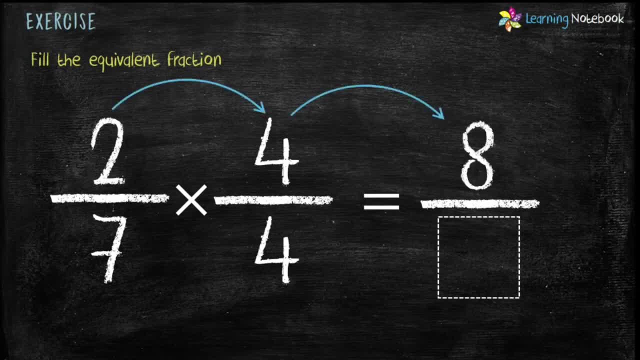 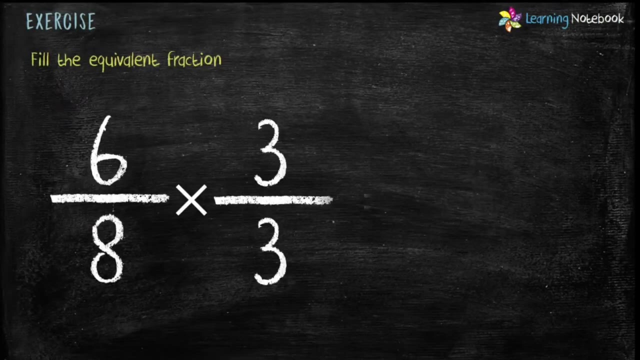 So numerator would be 2 into 4, equals to 8, and denominator would be 7 into 4, equals to 28.. Therefore, equivalent fraction is 8 by 28.. Now let's see another example. Here, numerator and denominator of fraction 6 by 8 are getting multiplied by same number, 3.. 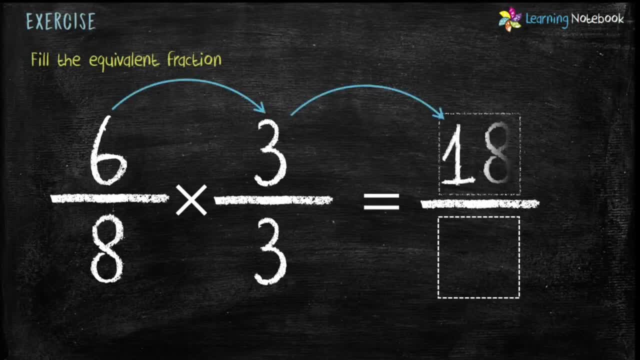 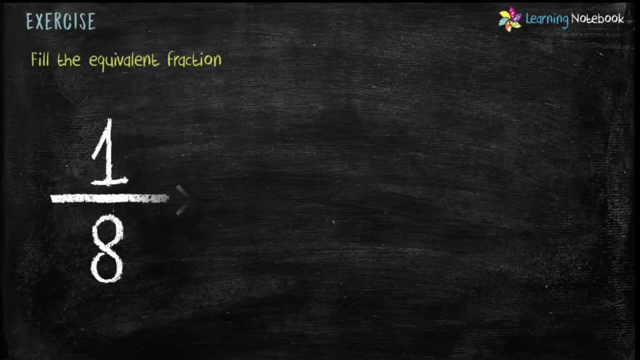 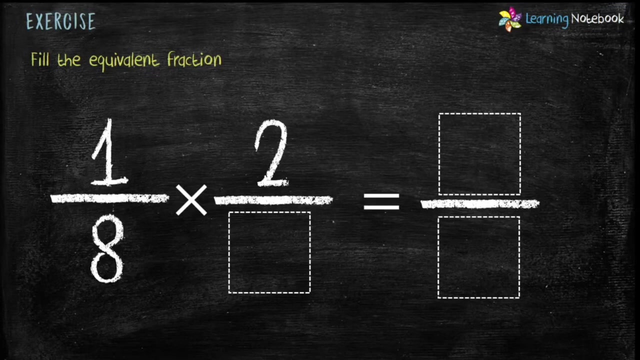 So numerator would be 6 into 3, equals to 18, and denominator would be 8 into 3, equals to 24.. So equivalent fraction is 18 by 24.. Let's see another example. Students, as we know, to make equivalent fraction, both numerator and denominator of a fraction should be multiplied by a same number. 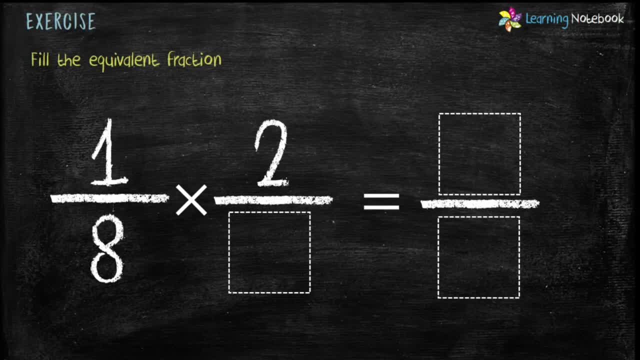 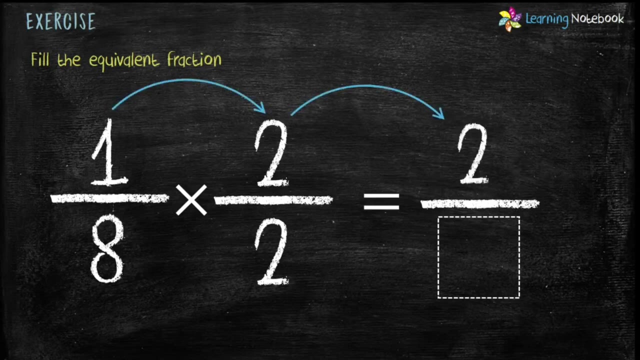 So in this example, numerator of fraction 1 by 8 is being multiplied by 2.. So denominator should also be multiplied by 2.. Now let's find the numerator of equivalent fraction. 1 into 2 equals to 2.. 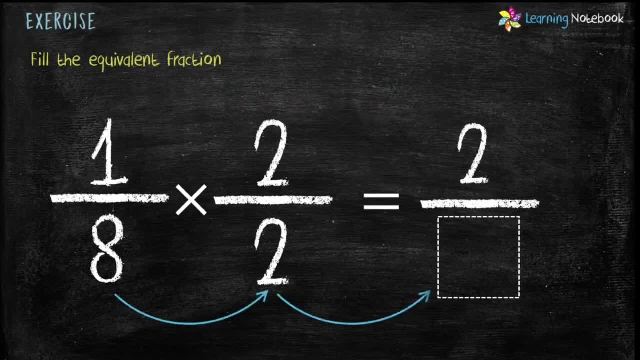 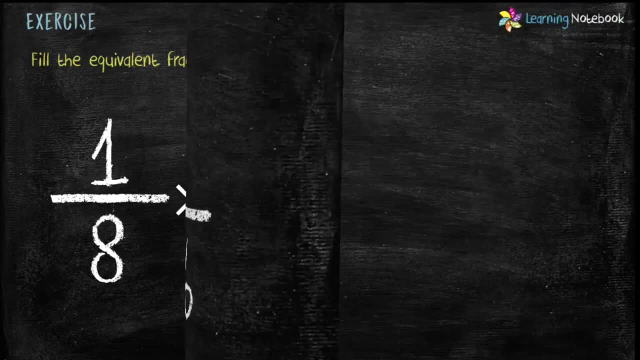 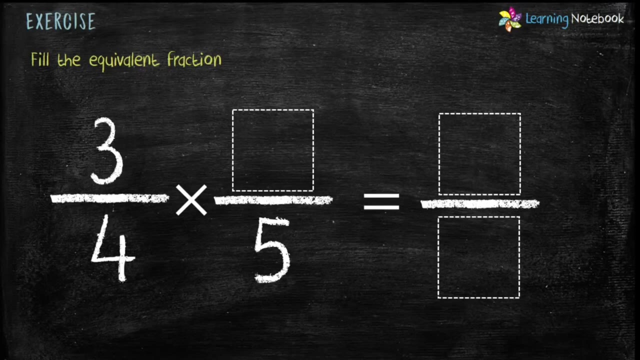 And its denominator would be: 8 into 2 equals to 16.. Therefore, equivalent fraction is 2 by 16.. Let's move to next question, Students, it is similar to the previous example. Now, in this example, denominator of fraction 3 by 4 is being multiplied by 5.. 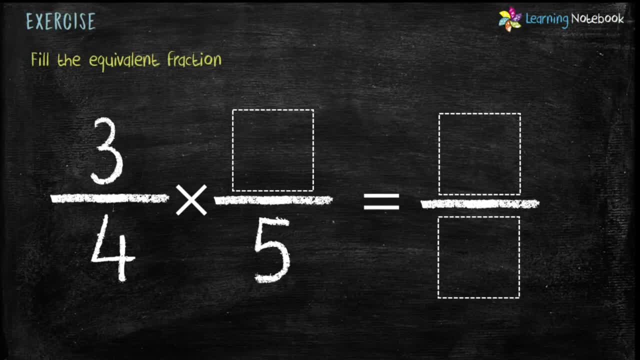 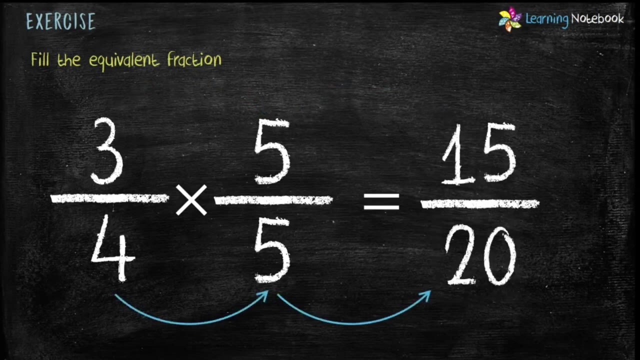 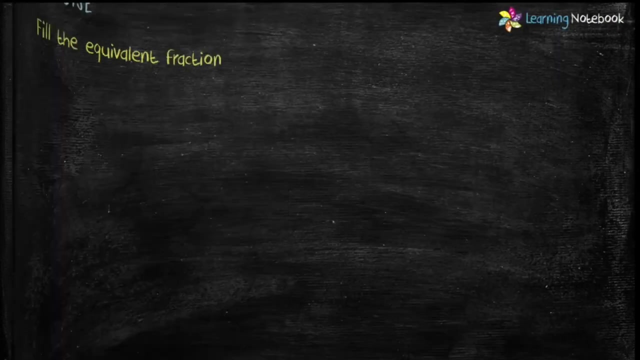 So numerator should also be multiplied by 5.. Now let's find the numerator of equivalent fraction. 3 into 5 equals to 15.. And its denominator would be: 4 into 5 equals to 20.. So equivalent fraction is 15 by 20.. 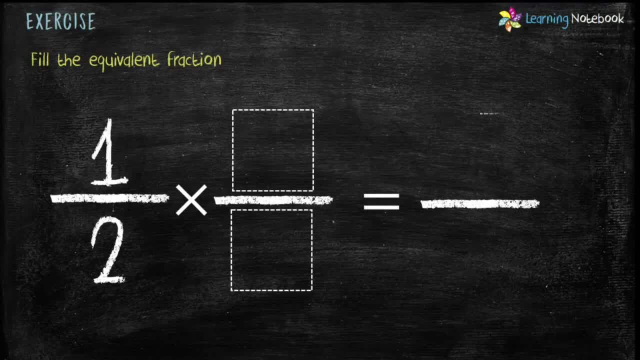 Now let's see next question, Students. in this question we first have to find out the number to be multiplied With both numerator and denominator of fraction, 1 by 2.. We are given denominators as 2 and 8.. 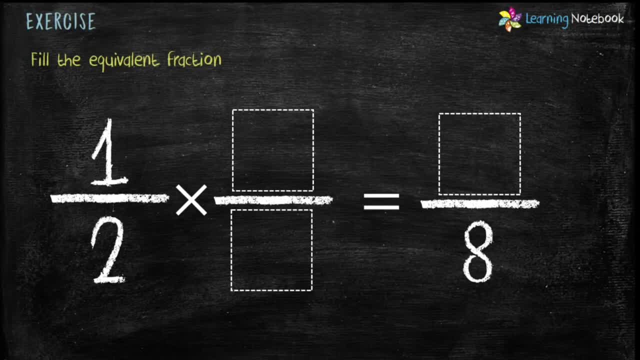 So, students, can you tell me what should be multiplied by 2?? So we get 8.. Yes, it is 4.. So 2 into 4 equals to 8.. Now we will multiply numerator and denominator. 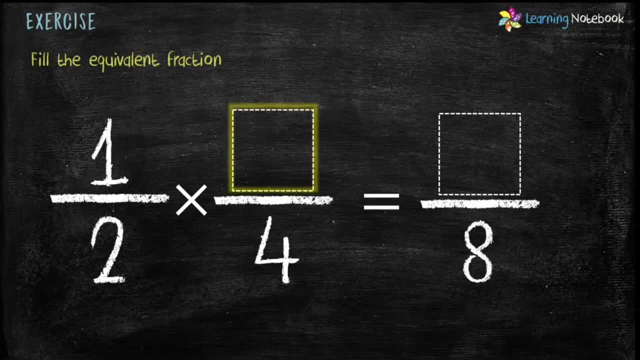 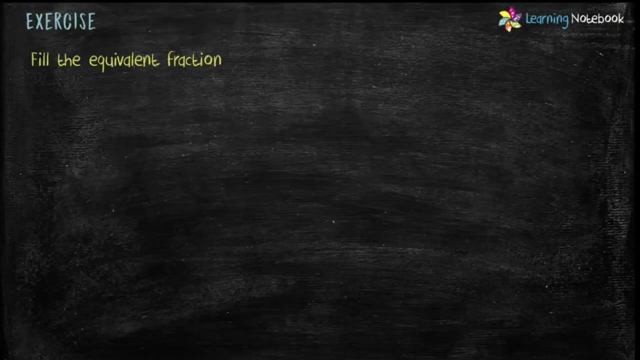 Numerator of fraction 1 by 2 with 4.. Therefore, numerator of equivalent fraction is: 1 into 4 equals to 4.. Therefore, equivalent fraction is 4 by 8.. Now, students, this is the next question. 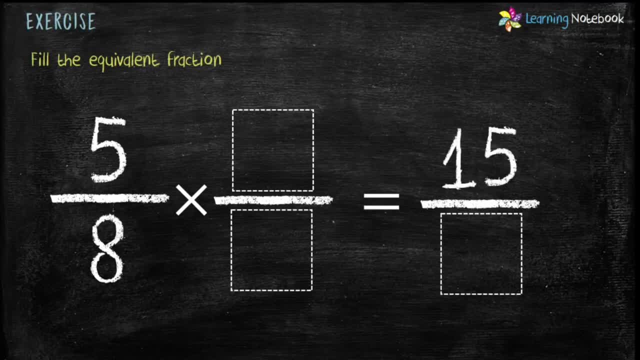 This question is similar to the previous question. We are given numerators as 5 and 15.. So which number should be multiplied by 5?? So we get 15.. Yes, it is 3.. As 3 into 5 equals to 15.. 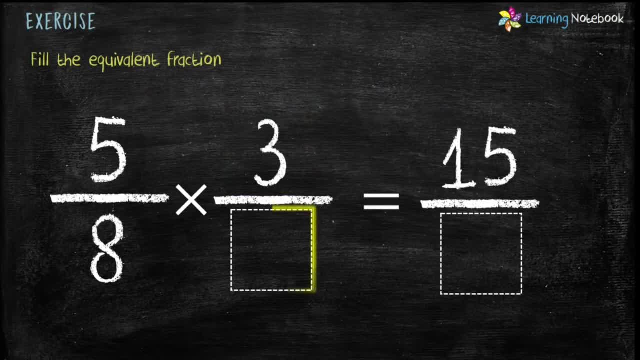 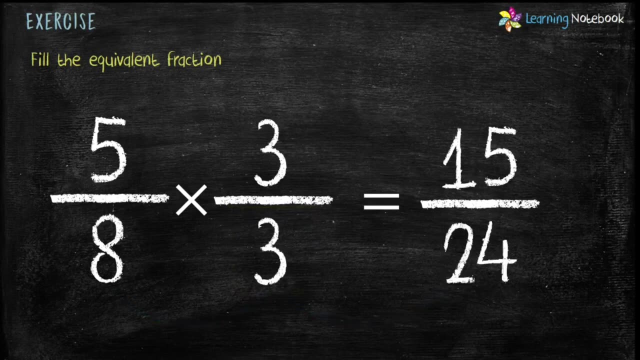 Now let's multiply numerator and denominator of fraction 5 by 8 with 3.. Therefore we get denominator of equivalent fraction as 8 into 3 equals to 24.. So, students, equivalent fraction is 15 by 24.. 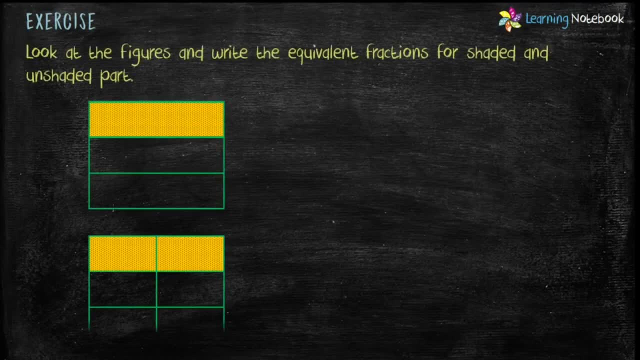 Let's move to next example. Look at the figures and write the equivalent fractions for shaded and unshaded part Students. in the first figure, fraction for shaded part is 1 by 3.. And in the second figure, fraction for shaded part is 2 by 6.. 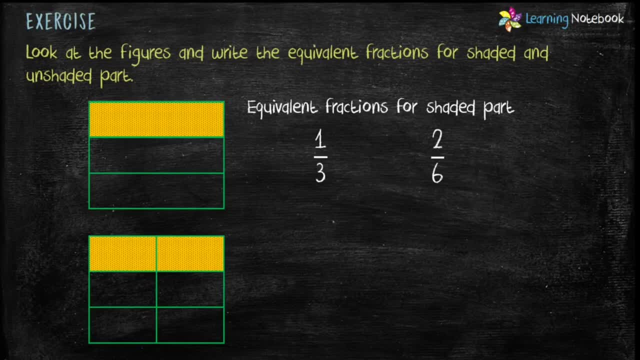 These fractions are equivalent fractions Because if you multiply numerator and denominator of fraction 1 by 3 with 2, we get 2 by 6.. Now let's see unshaded part In the first figure. fraction for unshaded part is 2 by 3.. 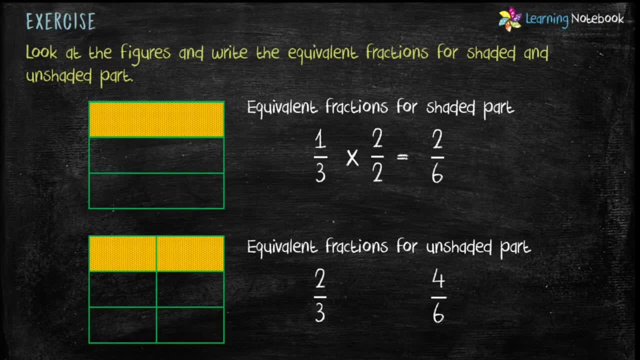 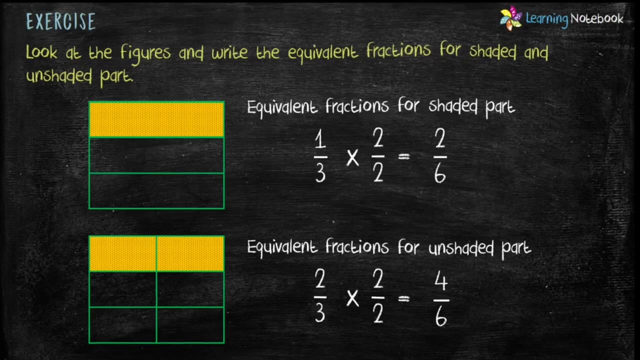 And in the second figure, fraction for unshaded part is 4 by 6. Again, these two are equivalent fractions, Because if we multiply numerator and denominator of fraction 2 by 3 with 2, we get 4 by 6.. 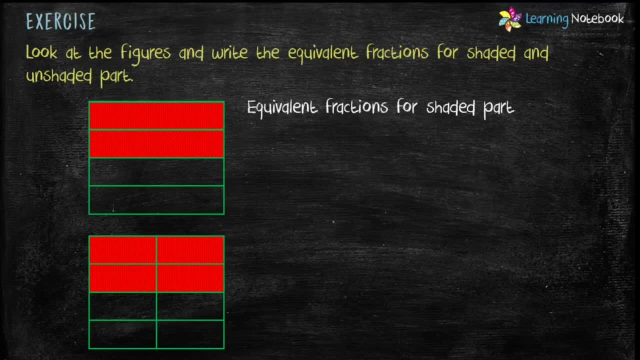 Let's do one more similar example. In the first figure, fraction for shaded part is 2 by 4.. And in the second figure, fraction for shaded part is 4 by 8.. These two fractions are equivalent fractions, Because if we multiply numerator and denominator of fraction 2 by 4 with 2, we get 4 by 8.. 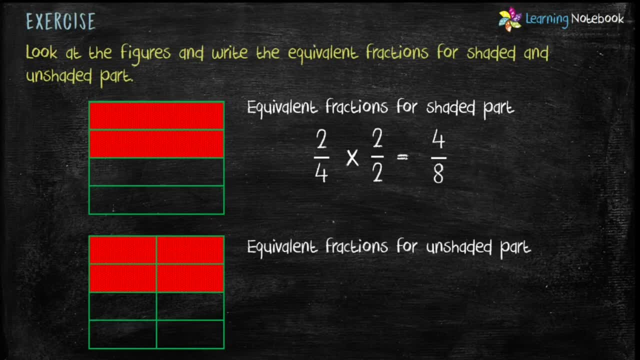 Now let's see unshaded part. Students, equivalent fraction for unshaded part is same as equivalent fractions for shaded part, Which is 2 by 4 into 2 by 2 equals to 4 by 8.. Now, students, this is our last example. 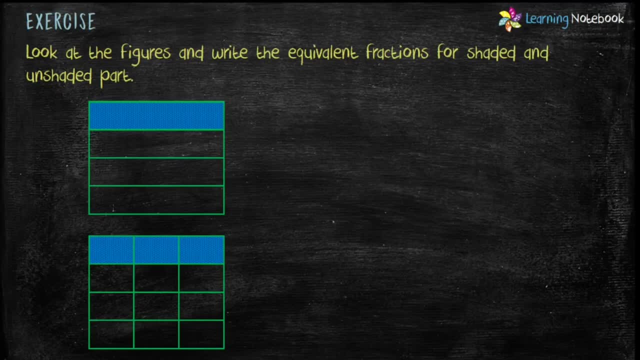 In the first figure fraction for shaded part is 1 by 4.. And in the second figure fraction for shaded part is 3 by 12.. And these two are equivalent fractions, Because if we multiply numerator and denominator of fraction 1 by 4 with 3, we get 3 by 12.. 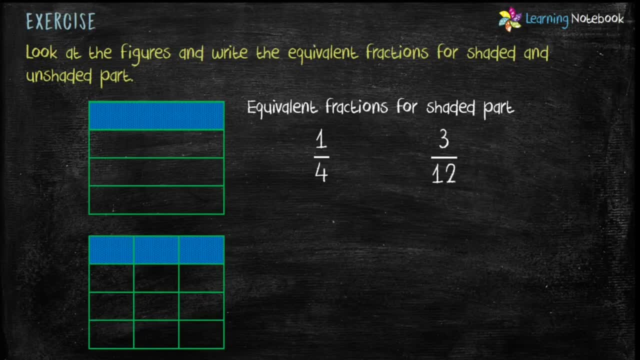 And these two are equivalent fractions, Because if we multiply numerator and denominator of fraction 1 by 4 with 3, we get 3 by 12.. Now let's see unshaded part In the first figure. fraction for unshaded part is 3 by 4.. 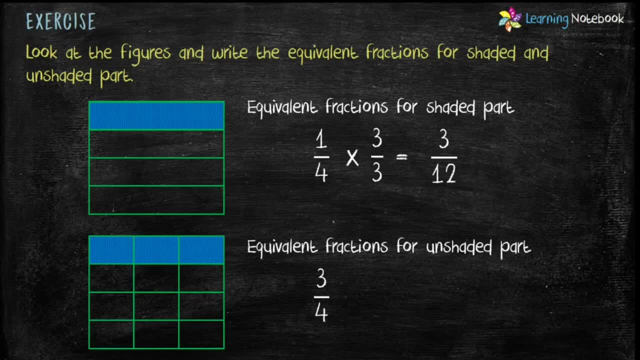 And in the second figure, fraction for unshaded part is 9 by 12.. Again, these two are equivalent fractions, Because if we multiply numerator and denominator of fraction 3 by 4 with 3, we get 9 by 12..